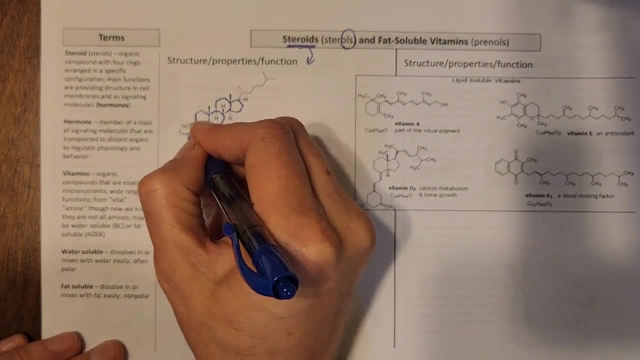 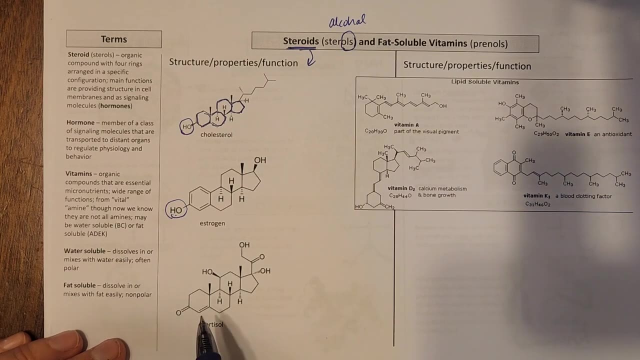 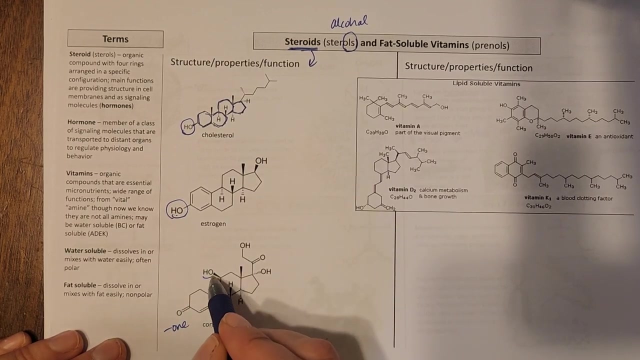 have this all At the end of them and you can see an alcohol that all is coming from, the alcohol that's present in these. Here's another alcohol. This cortisone or cortisol, has an own, a ketone, here at the end, but it does also have a few alcohol groups on it as well. So we're looking at steroids with the 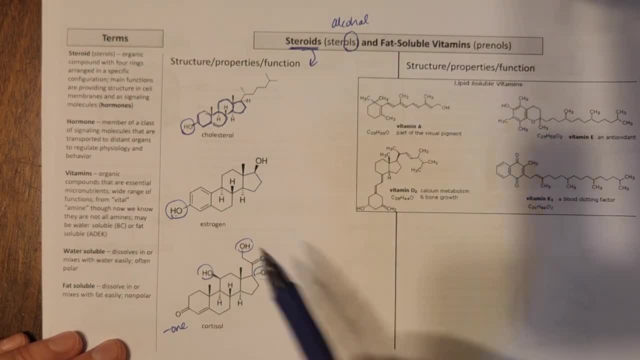 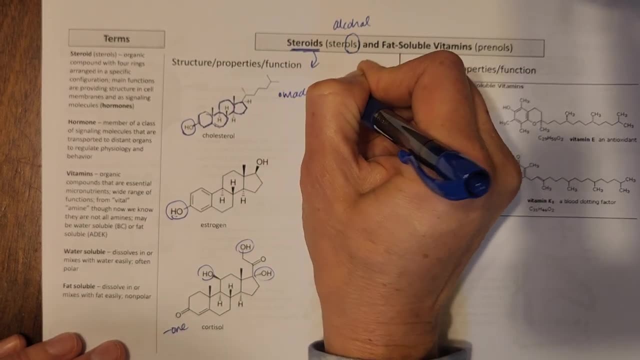 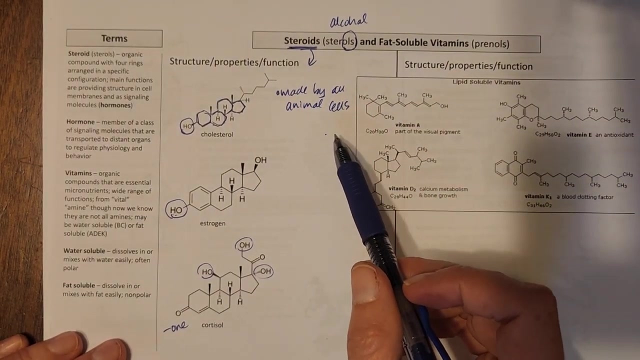 four fused rings and many of them have that alcohol, so they have that all ending. So, talking briefly about cholesterol, Cholesterol is made by all animal cells. So if you're trying to reduce your cholesterol, that's why sometimes nutritionists will say or physicians will say, you know, cut back on animal products. So 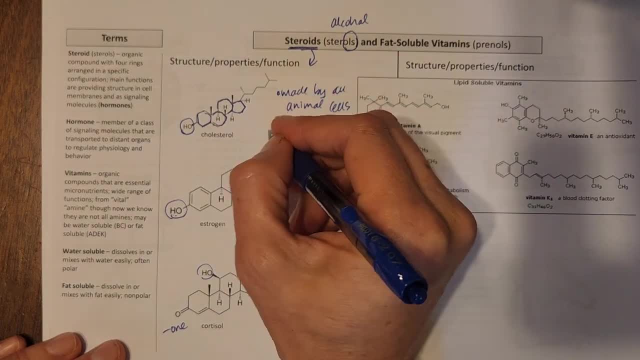 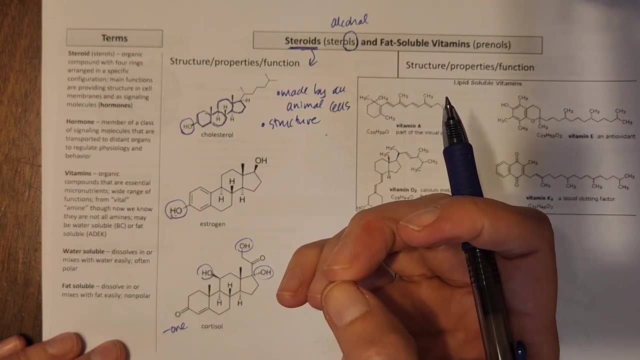 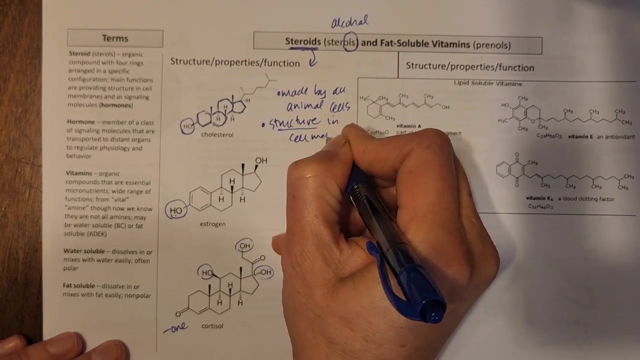 cheese and eggs and meat and things like that. These are cholesterol molecules are used for structure. So remember we've been talking about, do we use these different lipids for structure or for storage? So these are used for structure. So cholesterol is a cell membrane. 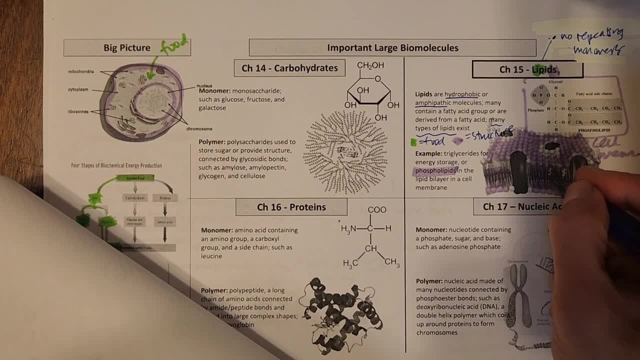 And if we can go back and look at a cell membrane picture, you can see in here some of these funny looking molecules. Those are cholesterols interspersed with the phospholipids. There's four rings there if you can barely see. So the cholesterols get embedded in the cell membrane to stiffen it up a. 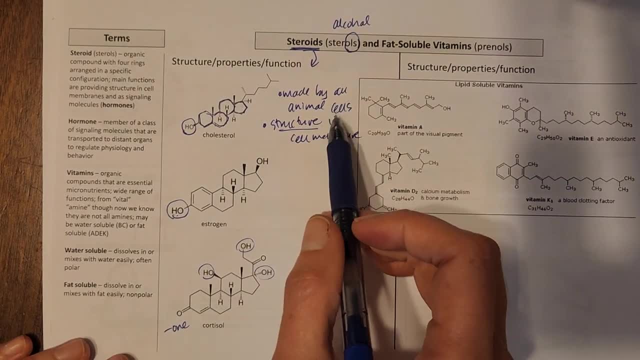 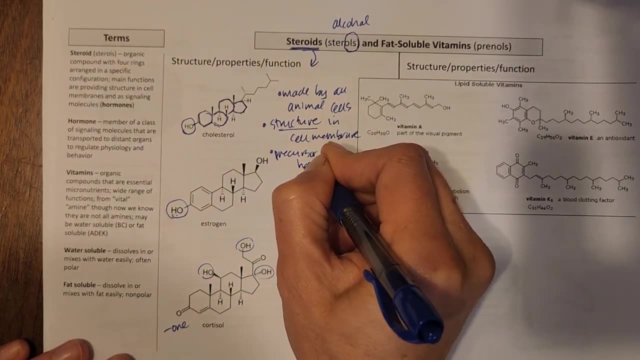 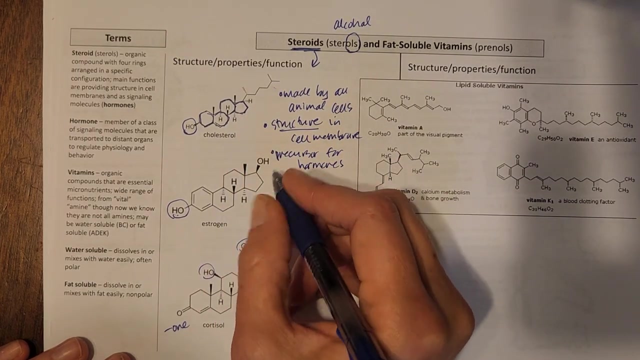 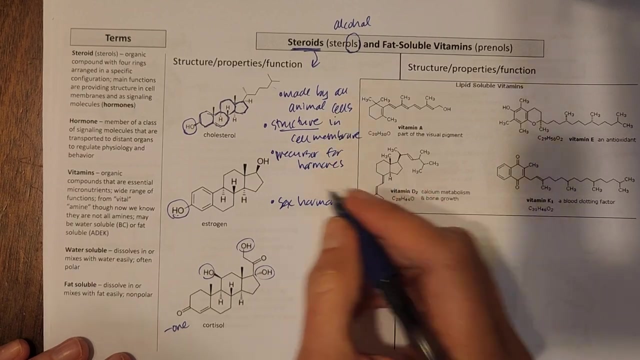 little bit so it is not quite so floppy. So that would be cholesterol. It's also a precursor for some of our hormones that we're going to see down below, So we would modify it and turn it into these. Estrogen is another example of a steroid. Our sex hormones are steroids. So this is an example of that and 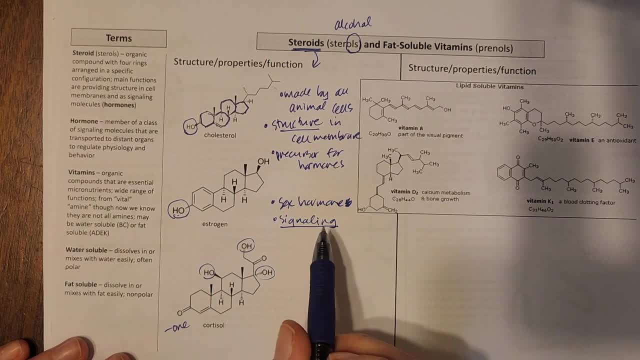 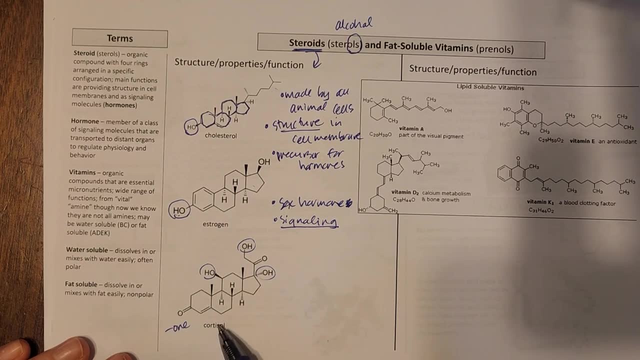 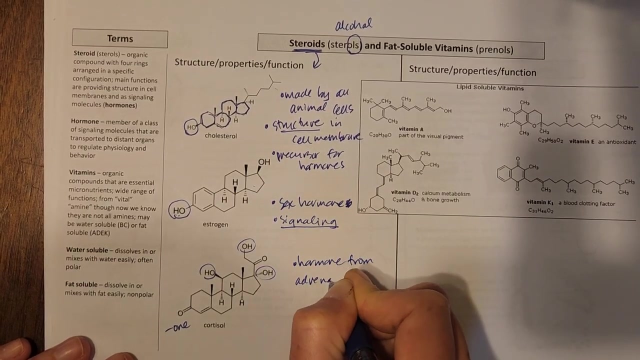 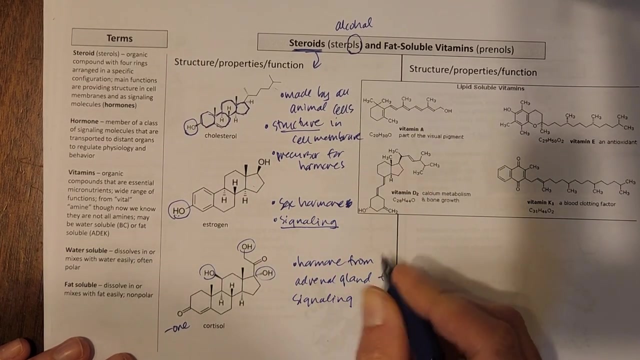 these would be used for something we haven't seen yet, which is signaling. So hormones are signalers, chemical signals, and that is what our sex hormones do. Last one to look at here, cortisol, is a hormone from the adrenal gland telling us how to act, how to feel. Again for signaling, And this will be signaling in. 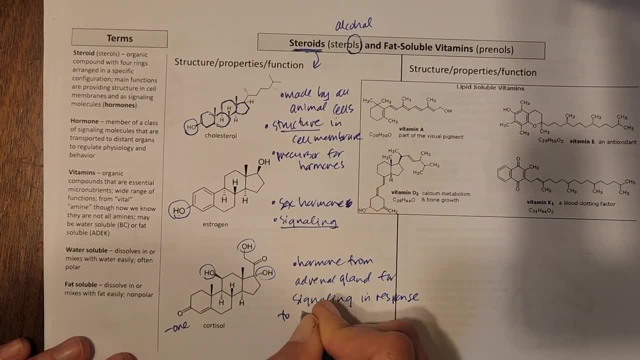 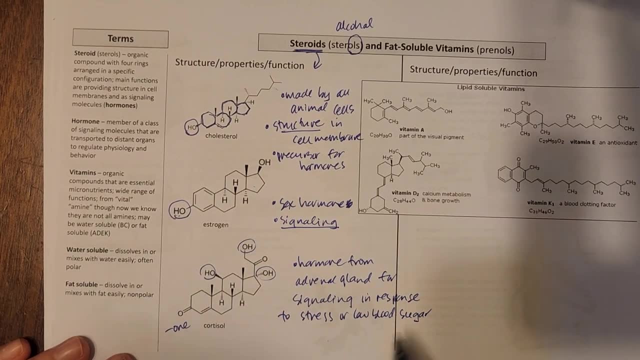 response to maybe two things you've experienced before: Stress, or also to low blood sugar. If you're hungry, there's a chemical reason why you're hungry. You've got steroids coursing through your body And so these are again good for signaling. 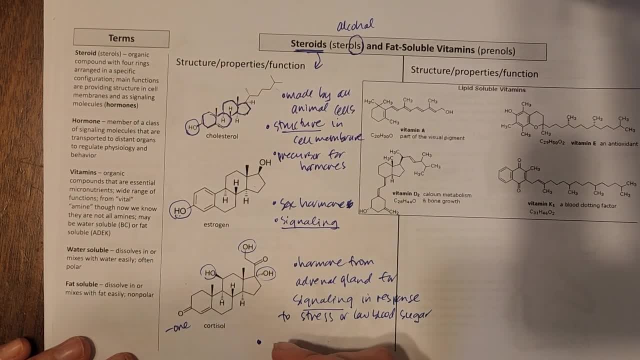 If we take the same chemical and we make it in a lab and we give it as a steroid medication, like a lotion you could get or an injection, this would go by a different name and its name would be hydrocortisone And that. 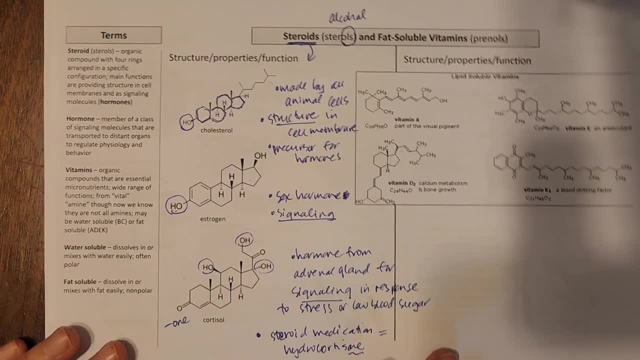 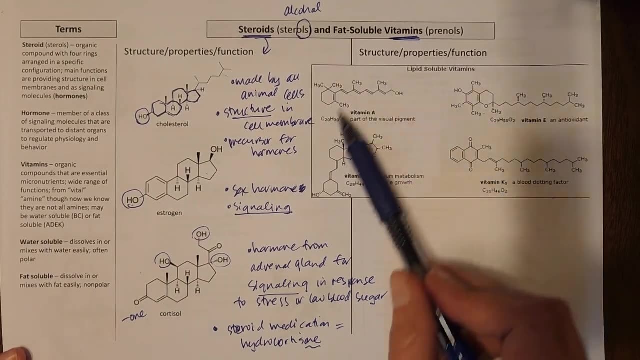 and that, at the end, comes from this ketone that I see right here. Let's see that. So then, over here, our final lipid we're going to look at is vitamins. So we have the lipid soluble, or fat soluble, vitamins here. These are: 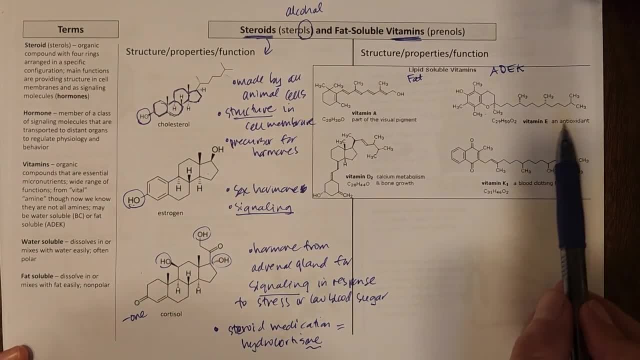 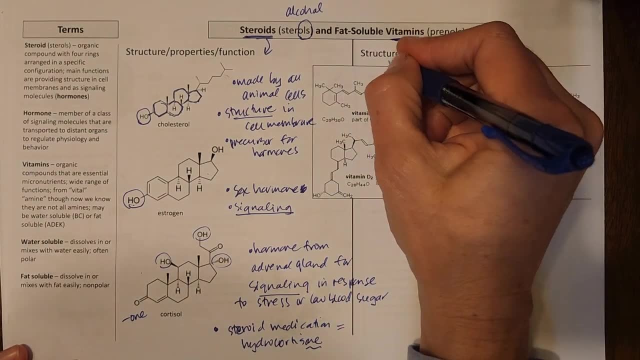 um A, D, E and K. If I look at all of these vitamins, you'll notice they're almost entirely C's and H's, So non-polar, Okay. Um, if you look at the water soluble vitamins, you'll see a lot. 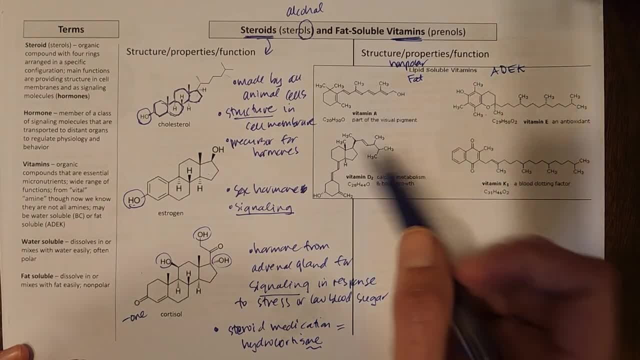 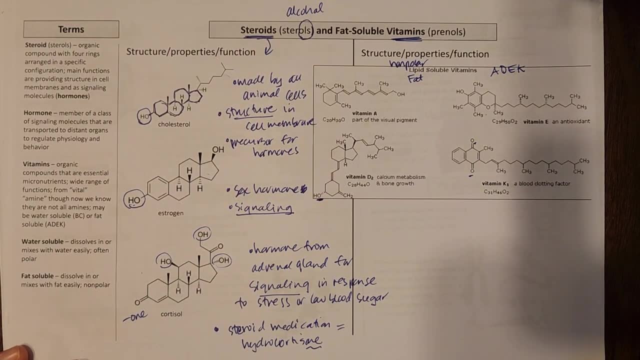 of hydroxyls, OHs on them, Um, but not here. Maybe you see one, maybe you see a couple oxygens, but relative to the 20 other carbons, these are very non-polar. Okay, So we could say that. 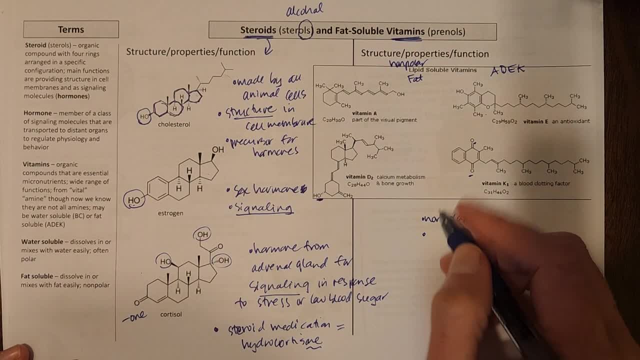 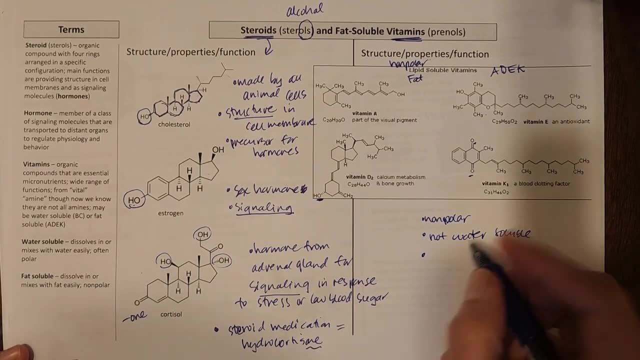 their structures are non-polar. As a result, their properties come out of that. We could say that they are not water soluble And finally, instead, we could put it in a positive light. These are fat soluble, which means you don't have to eat them constantly. Your body stores up a bit. 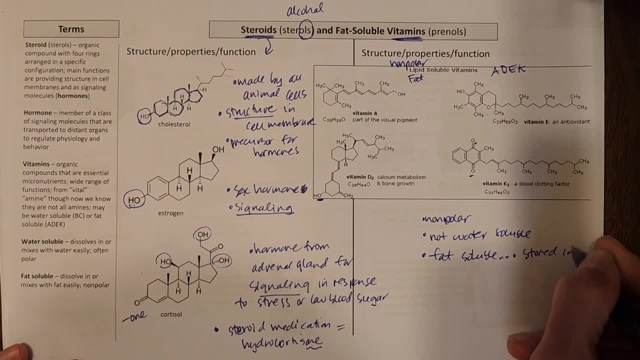 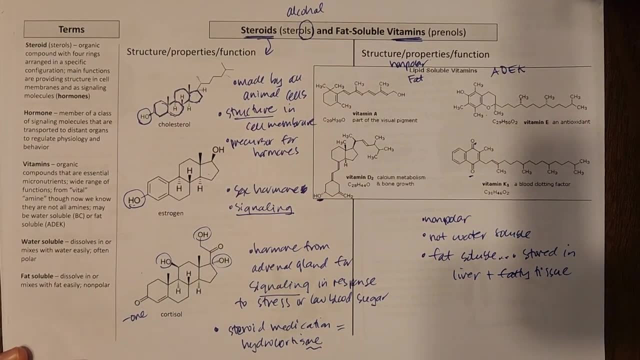 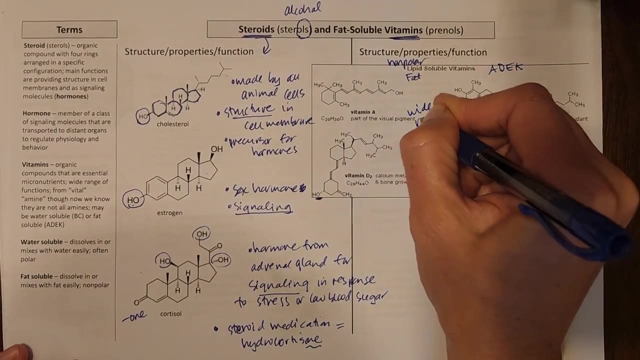 of supply, Um, so these will be stored in your liver and in fatty tissue, And so that you can tap into them, um as needed. Okay, So those are the two things that we're going to talk about today. Those? um vitamins tend to have a really wide range of uses, Um, but structure is one of the. 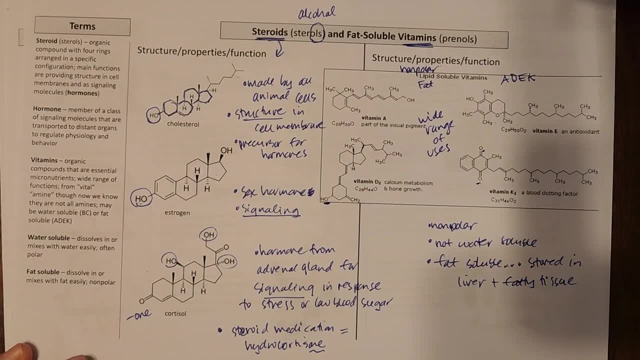 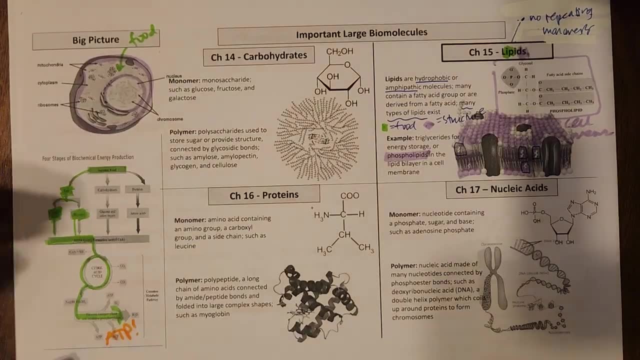 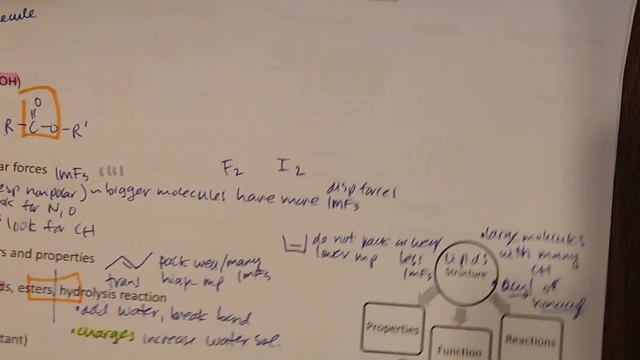 uses for them. They're also precursors for a lot of other processes, things like coenzymes in our body, Um, so that is a glimpse of our steroids and our vitamins. If we come back to the beginning of our day, um, we had talked about the structure and function and properties and reactions. um,